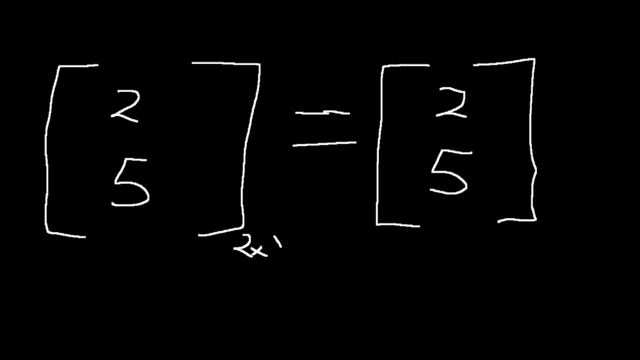 equal, because each element matches. But where it becomes interesting with equality is you can have a formula or a function on one side and a result on the other, and then it essentially turns into an algebra equation, Something like: well, maybe you'll have 7x here and let's change these two. 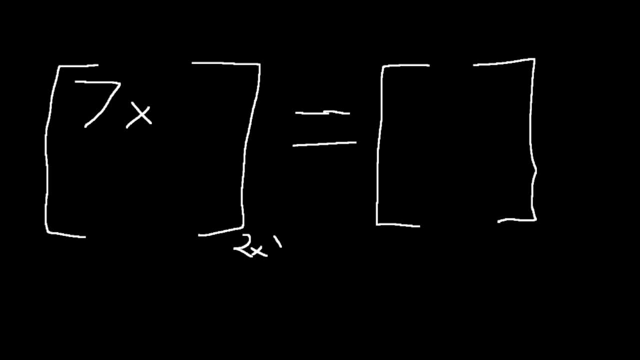 Maybe you have 7x plus 1 as this first element here in row 1, column 1, and over here we have 15, and let's put another random thing down here, Like 9 plus 2y, and over here maybe we'd have another 15.. So from this, since it tells us, they're. 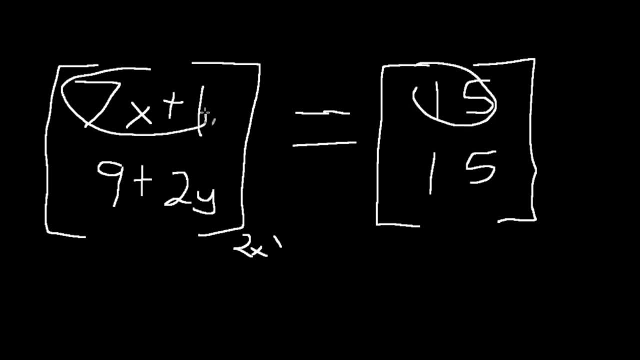 equal. we know that this element here is the same as this element here, which would allow us to solve for x. So it would turn into this: And of course, x here would be 2, because 7 times 2 is 14, plus another 1 is 15.. And likewise for: 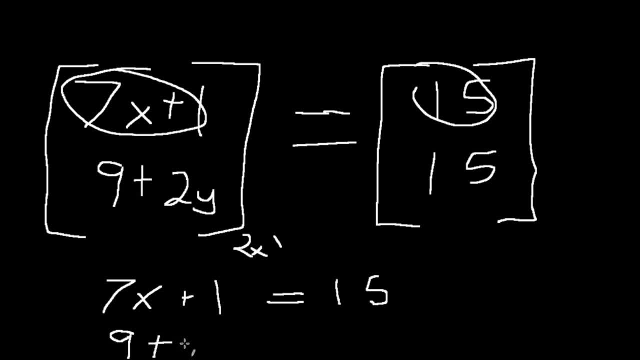 this bottom one, we could do the same thing. We know that they're equal. we could set it up like so: And in this case, what would this y be? See, if you can figure that one out on your own, It's 3.. 9 plus 6 equals 15.. So y would be 3.. So that's how equality works. It's just element by element. 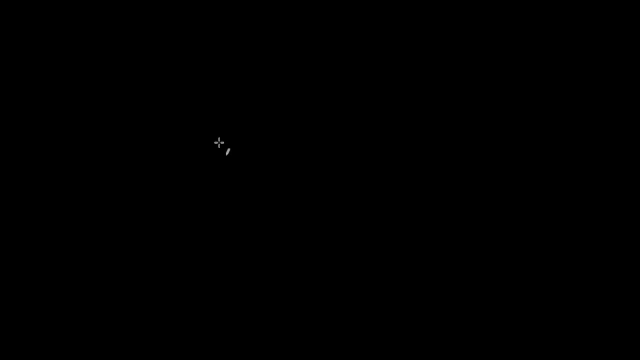 And now let's talk about addition and subtraction. To add or subtract matrices, they need to be the exact same size. Let's say these are each 2 by 2.. I'll just put 2 by 2 down here. Random numbers, That's an 8, 1, and a 9, and a 10.. 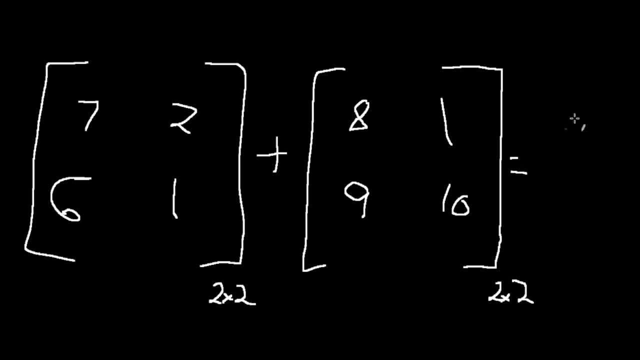 And this would equal a- I'm running out of room here- a matrix of the same size where each element is just added together. Or, for this first one, it would be a matrix of the same size where each element is just added together. 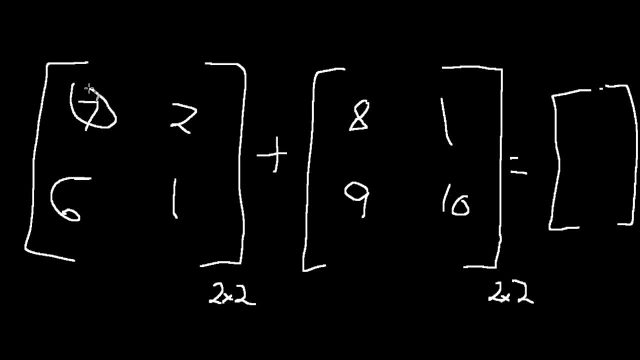 Or for this first one, it would be a matrix of the same size, where each element is just added together. And the next one is 2 plus 1,, which is of course 3. And then 6 plus 9,, which is of course 15.. 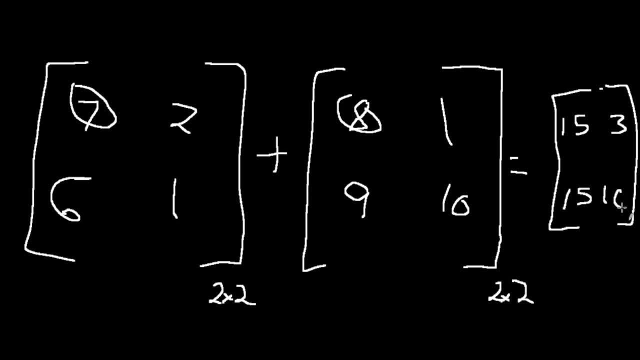 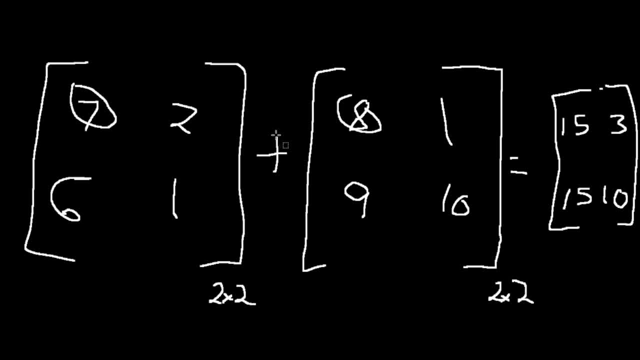 element by element. So I think you can figure that out on your own. It is important that they are the same size, or you just can't do the operation and it is an illegal try. So one last thing here is these: do follow the standard rules of 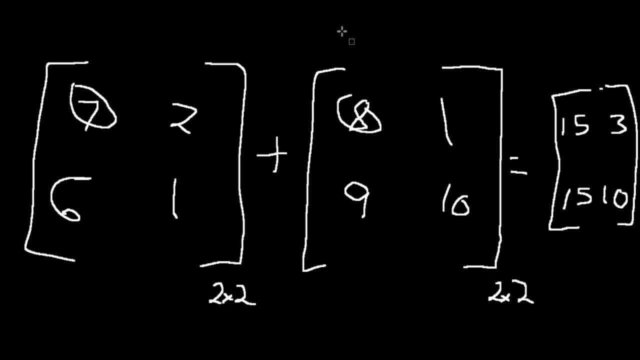 addition and and subtraction where they are communitive and associative, And basically what that means is the order of them doesn't matter. So you could put this matrix first and this one second, and they would equal the same thing. Or if you added a third matrix in here that was 2 by 2 to add to it, you would just 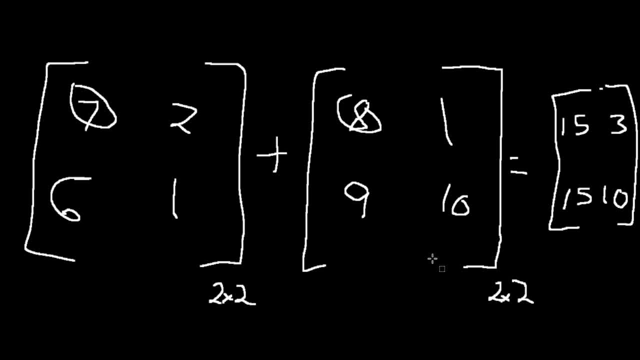 keep adding up the results, And the order, of course, doesn't matter. Okay, that's going to do it for this episode. Please leave a like and check the links below to help support this channel If you'd like to see more videos, higher quality videos, etc. etc. I'm a young, growing channel, A young growing boy in 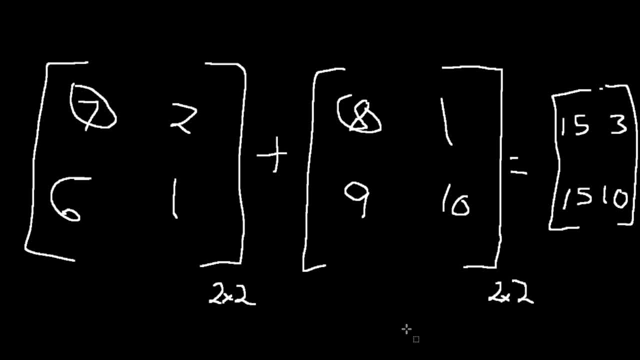 the YouTube world, So I could use any support that I could get. Have a good day and keep on growing, Learning guys.